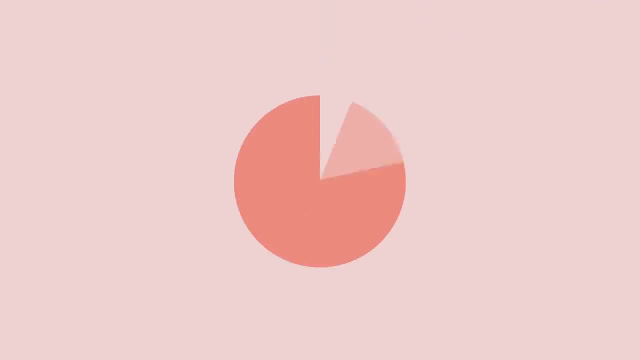 these methods were no longer sufficient. So, as they developed, different civilizations came up with ways of recording higher numbers. Many of these systems, like Greek, Hebrew and Egyptian numerals, were just extensions of tally marks, with new symbols added to represent larger magnitudes of value. Each symbol was repeated as many times as necessary. 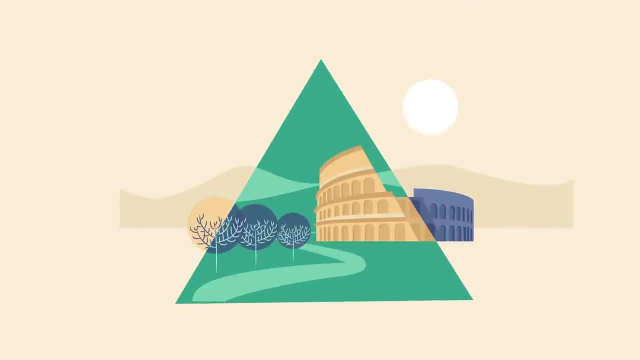 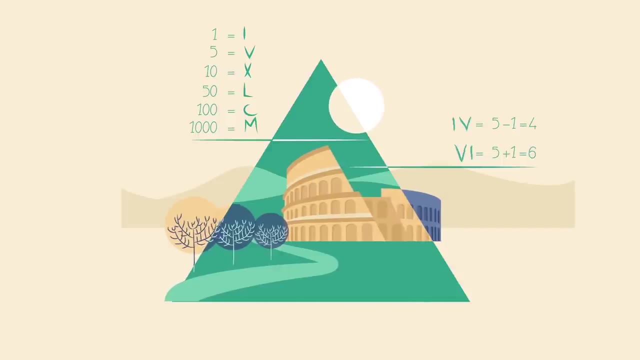 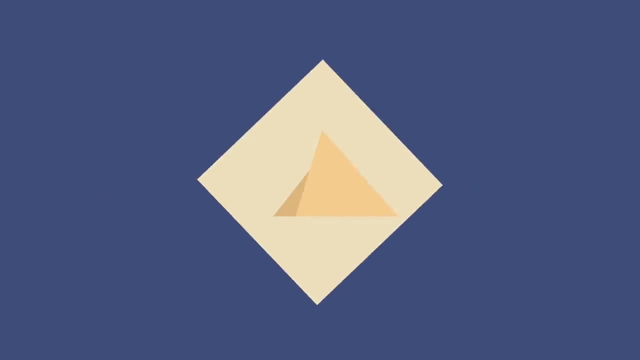 and all were added together. Roman numerals added another twist: If a numeral appeared before one with a higher value, it would be subtracted rather than added. But even with this innovation it was still a cumbersome method for writing large numbers The way. 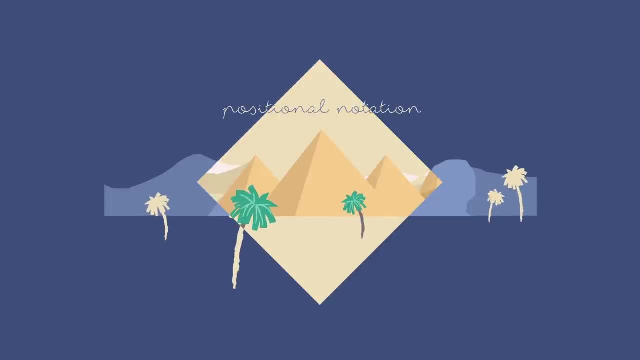 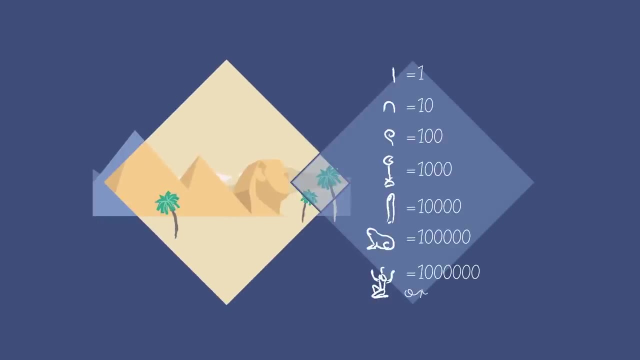 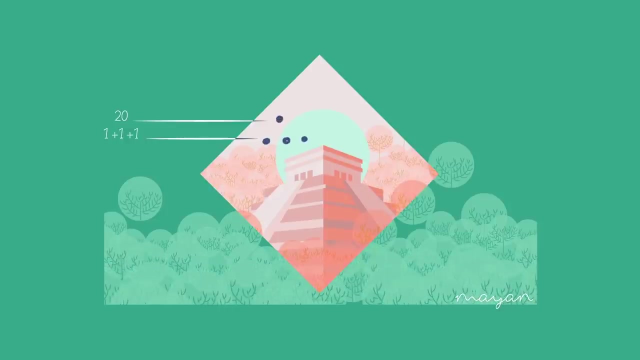 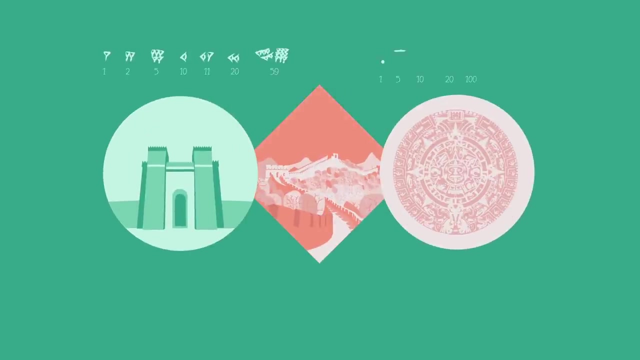 a useful and elegant system lay in something called positional notation. Previous number systems needed to draw many symbols repeatedly and invent a new symbol for each larger magnitude, But a positional system could reuse the same symbols, assigning them different values based on their position in the sequence. Several civilizations developed positional notation. 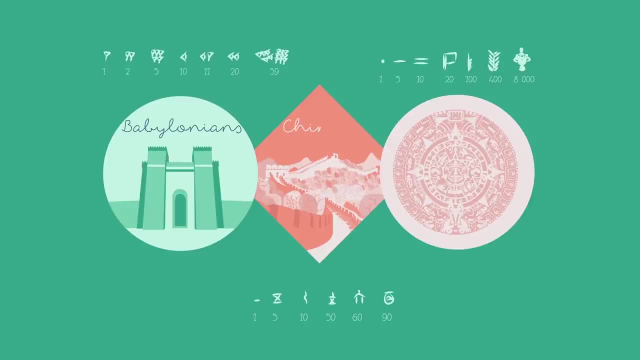 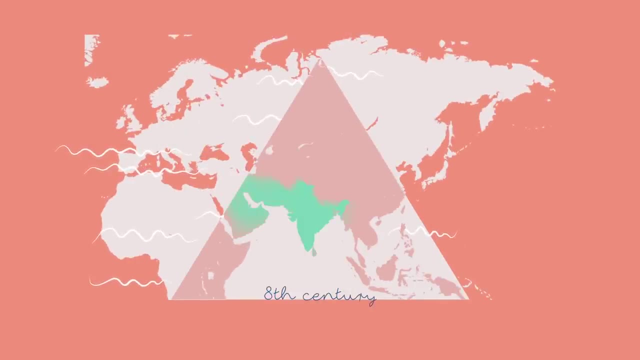 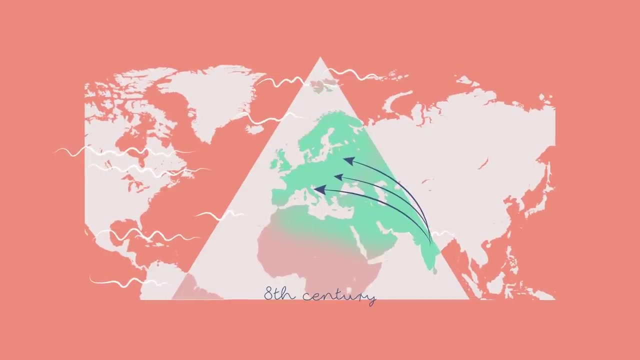 independently, including the Babylonians, the ancient Chinese and the Aztecs. By the 8th century, Indian mathematicians had perfected such a system and over the next several centuries, Arab merchants, scholars and conquerors began to spread it into Europe. 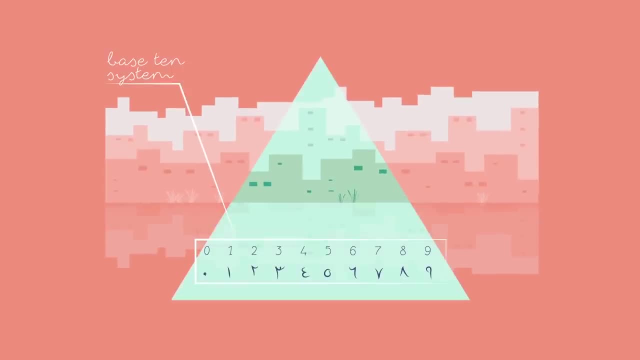 This was a decimal or base-10 system which could represent any number using only 10 unique glyphs. The positions of these symbols indicate different powers of 10, starting on the right and increasing as we move left. For example, 616 reads as: 6 times 10 to the zeroth power plus 1 times 10 to the first power plus 3. 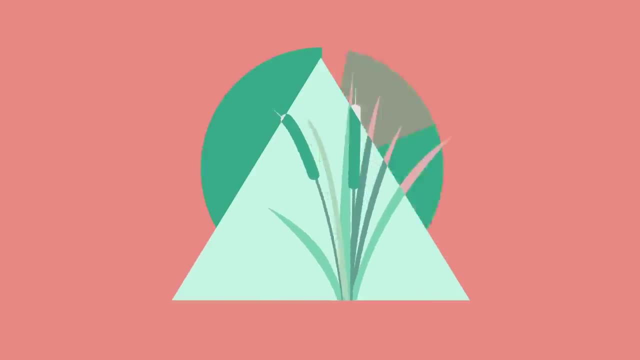 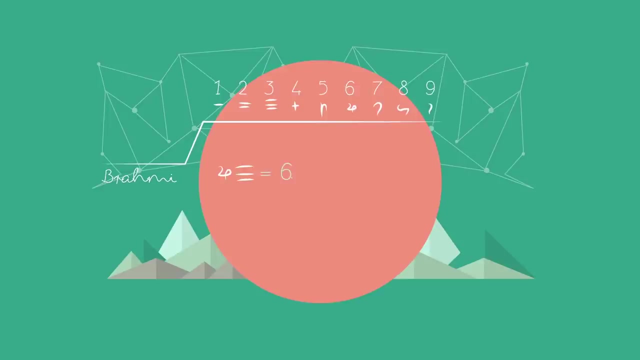 times 10 to the second power. A key breakthrough of this system, which was also independently developed by the Mayans, was the number zero. Older positional notation systems that lacked this symbol would leave a blank in its place, making it hard to distinguish between 63 and 603, or 12 and 120. 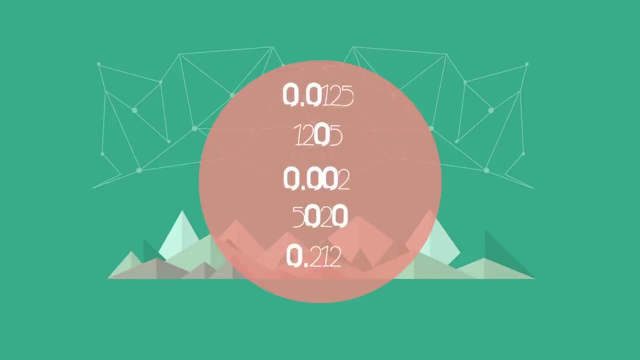 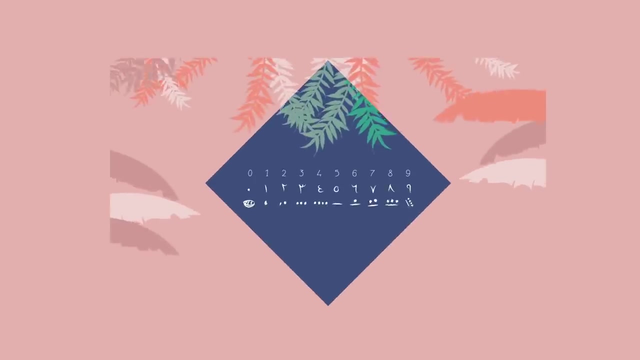 The understanding of zero as both a value and a placeholder made for a reliable and consistent notation. Of course, it's possible to use any 10 symbols to represent the numerals zero through nine. For a long time, the glyphs varied regionally. 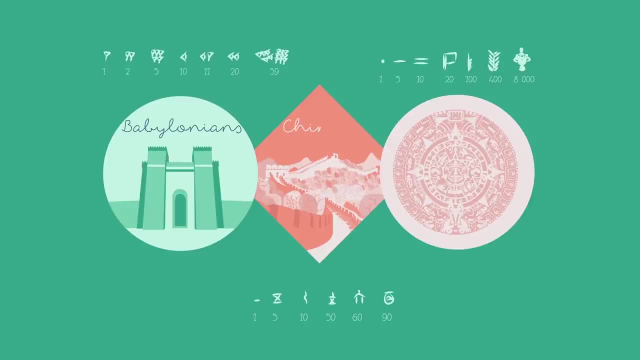 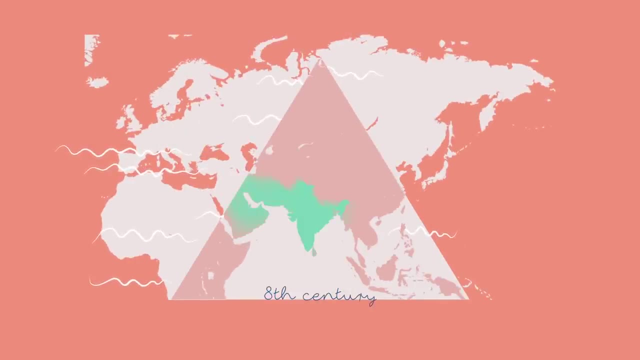 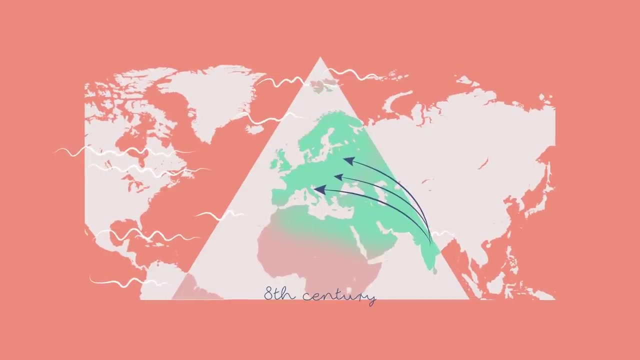 independently, including the Babylonians, the ancient Chinese and the Aztecs. By the 8th century, Indian mathematicians had perfected such a system and over the next several centuries, Arab merchants, scholars and conquerors began to spread it into Europe. 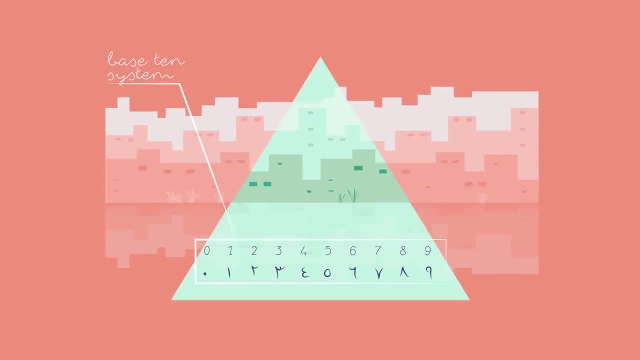 This was a decimal or base-10 system which could represent any number using only 10 unique glyphs. The positions of these symbols indicate different powers of 10, starting on the right and increasing as we move left. For example, 616 reads as 6 times 10 to the zeroth power, plus 1 times 10 to the first power. 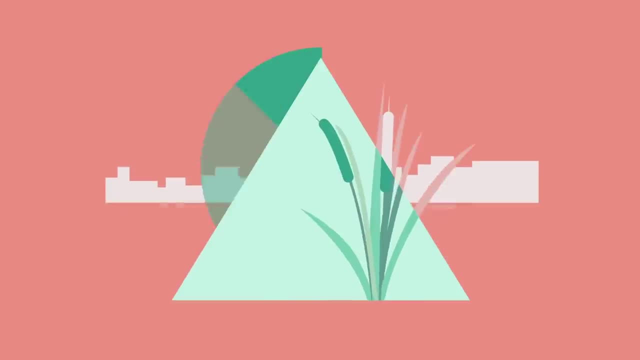 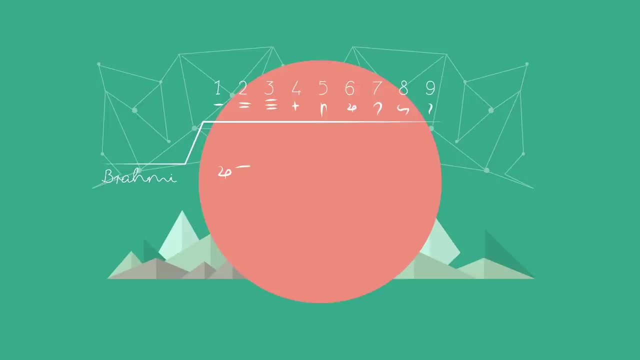 plus 3 times 10 to the second power. A key breakthrough of this system, which was also independently developed by the Mayans, was the number zero. Older positional notation systems that lacked this symbol would leave a blank in its place, making it hard to distinguish between 63 and 603, or 12 and 120. 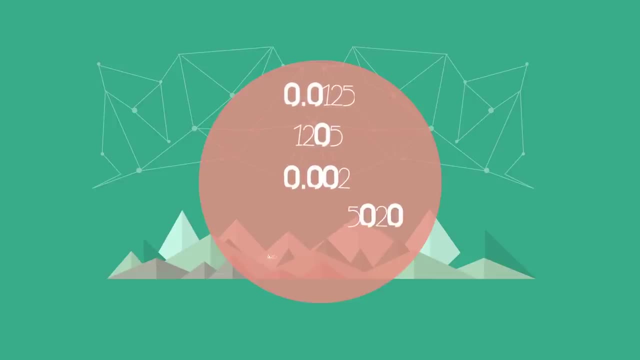 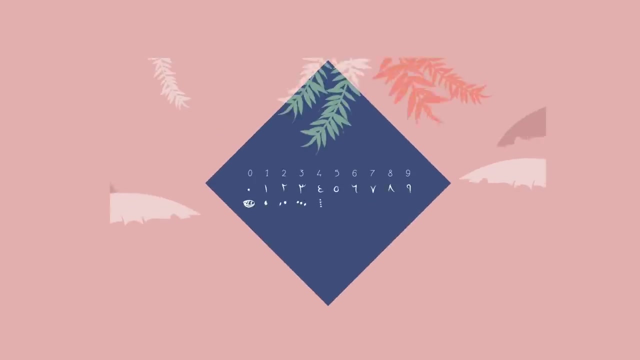 The understanding of zero as both a value and a placeholder made for a reliable and consistent notation. Of course, it's possible to use any 10 symbols to represent the numerals 0 through 9.. For a long time the glyphs varied regionally. Most scholars agree that our current digits 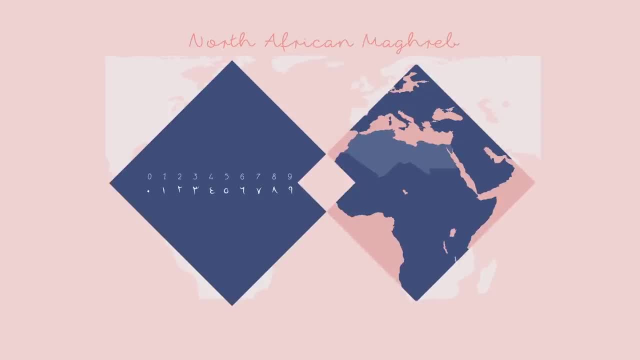 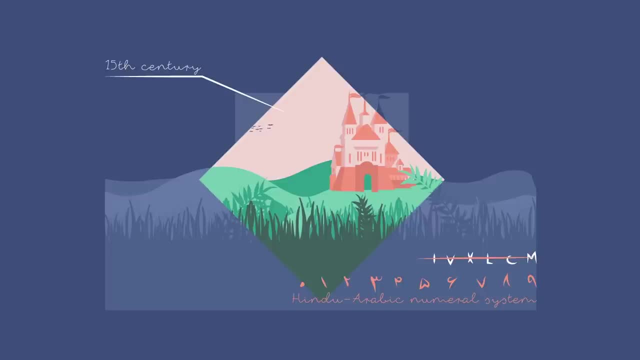 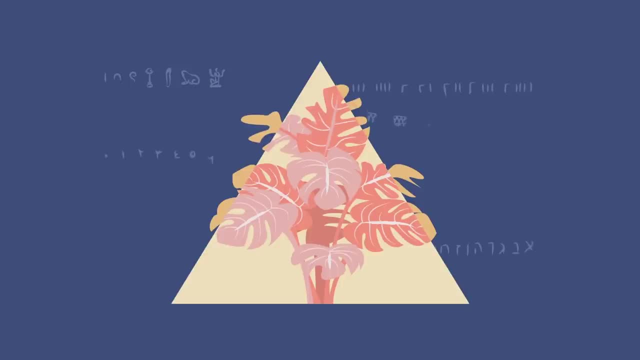 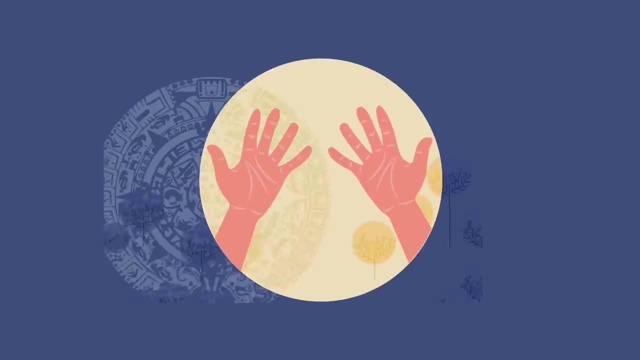 So why did the Hindu-Arabic system, along with so many others, use base-10?? The most likely answer is the simplest. That also explains why Aztecs used base-20, or Vage-steimal system – notes below. But other bases are possible too. Babylonian numerals were sexage-så-mal or base-sixty, And many people think that a base 12, or duodecimal system would be a good idea. Like 60,, 12 is a highly composite number that can be divided by 2,, 3,, 4, and 6,.